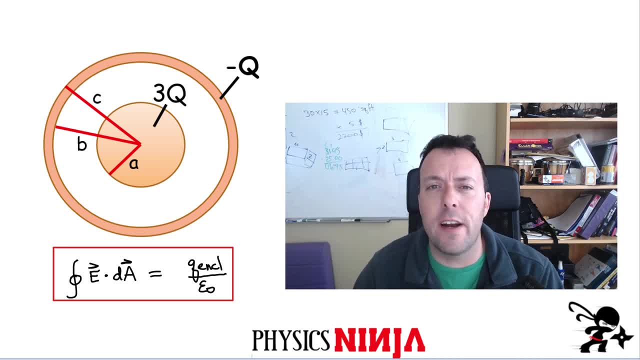 And the geometry I'm considering here is the one shown in the figure. So what we have here is a sphere at the center of a shell. So the sphere- the inner sphere- has a radius A, the outer shell has a thickness, and the inner radius is B and the outer radius is C. 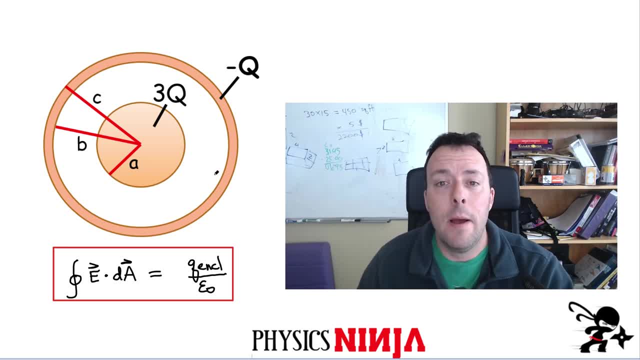 So how would you solve for the electric field everywhere in space? And what we're going to do is we're going to consider two cases. So case number one, for this inner sphere- I'm going to assume that it is a conductor- And again, that inner sphere has a total charge equal to 3Q. 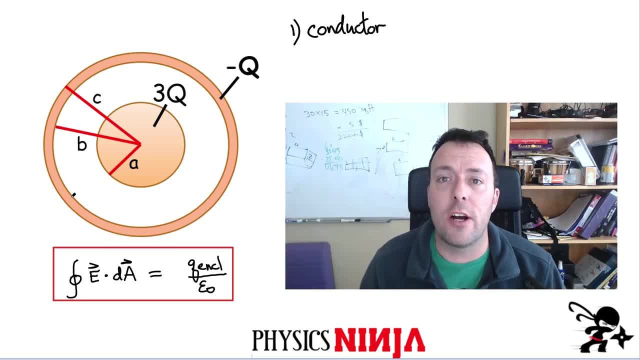 The outer shell has a total net charge of negative Q. So how would you set up Gauss's Law to solve for the electric field everywhere? And for the second case, what I'm going to do is I'm going to assume that this inner sphere is an insulator and the charge is uniformly distributed throughout the volume of that sphere. 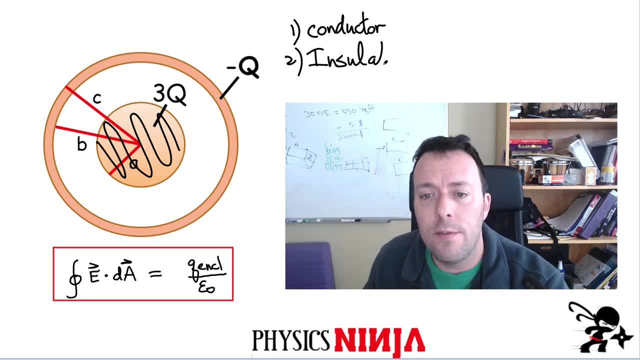 So we've got two different cases. If it's insulating versus conducting, what is the difference? How do you set up Gauss's Law? What makes it different? All right, so let's get started Again. if you liked the video, give it a thumbs up. 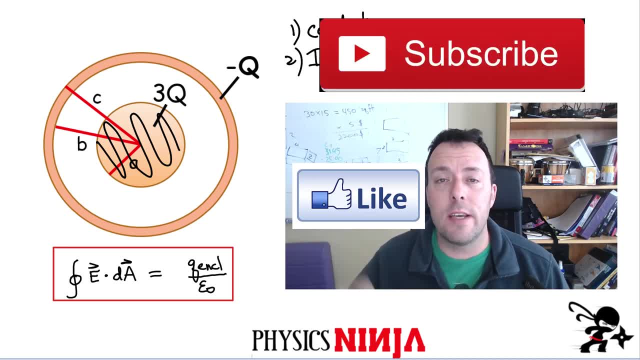 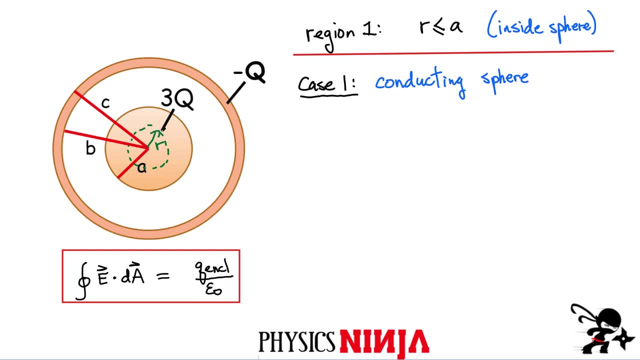 Consider subscribing to my channel, And if you have any questions, leave them in the comments section. I'll get back to you. Okay, so case one here is the case where we're gonna assume that this inner sphere is conducting Okay and my goal is to find the electric field. 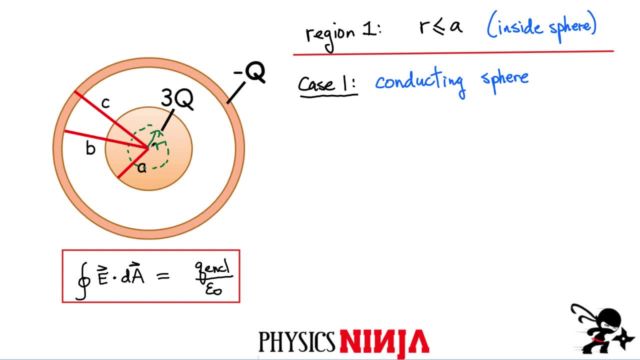 in region one, so anywhere within this sphere. So the first thing you do for case one is, if it's a conducting sphere, Okay. this is a very, very special word. If you hear that word conducting sphere, it means by definition, okay. 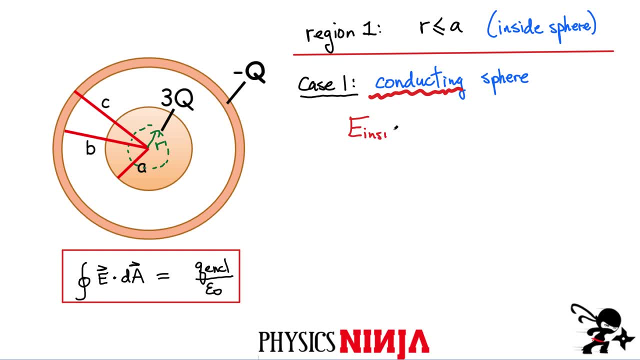 that the electric field inside must be equal to zero. Well, how is that possible? Okay, the only way that it's possible from Gauss's law that you get zero, the only way that's possible is if the enclosed charge of my Gaussian surface 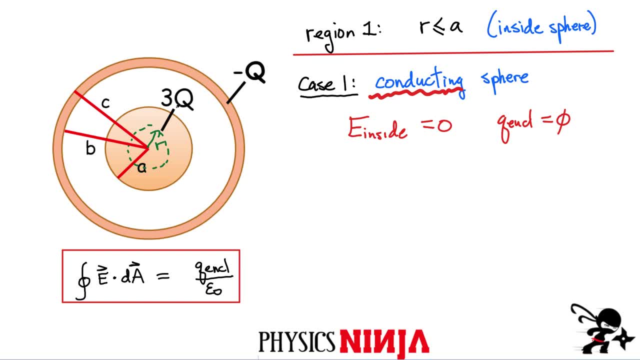 also equals to zero. So what that means here is that this 3Q must be spread out evenly on this spherical surface. Okay, so this is what's going to happen for a conductor: You can't have any charge anywhere inside, because that would produce an electric field. 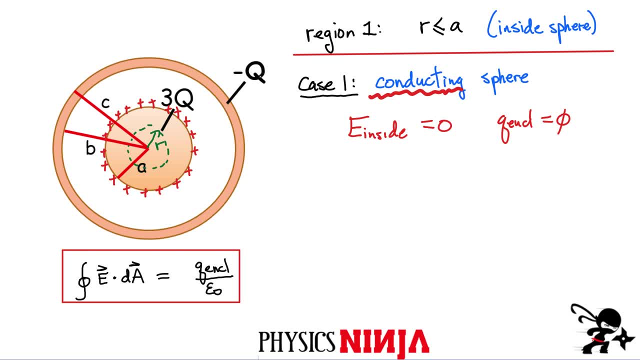 and then that means that the charges would move because there'd be a force acting on them. Okay, so case one is kind of just a definition that the field inside a conductor must be zero, so all of the charge is going to be on the outside. 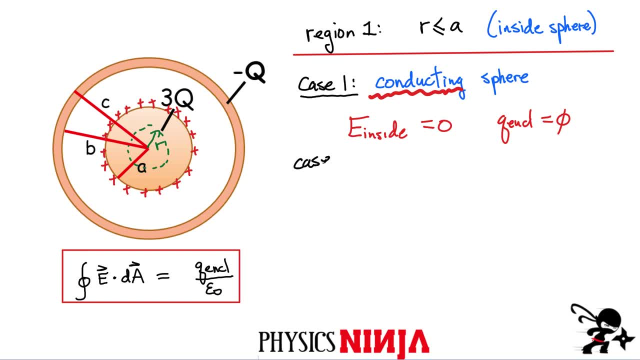 Okay, now, case two is a little bit more complicated. So for case two, what we're going to assume is that: okay, so case two is a little bit more complicated. So for case two, what we're going to assume is that: 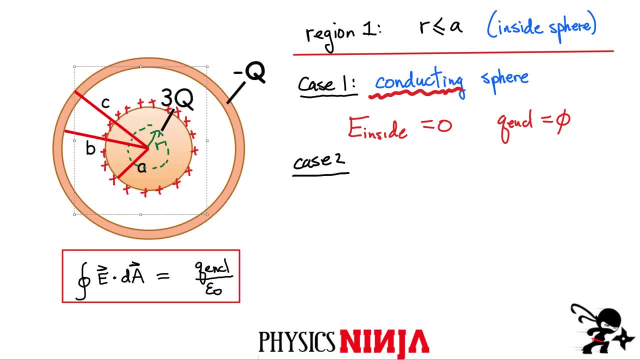 okay, so case two is a little bit more complicated. So for case two, what we're going to assume is that the charge is going to be uniformly distributed throughout the entire volume here of right. we're going to assume that it's uniformly distributed. 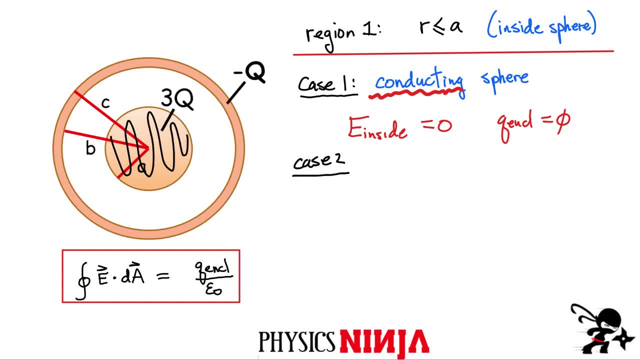 throughout the entire volume of this sphere. Okay, so what we have to do now is: now you really have to apply Gauss's law for this. So the first thing we're going to do is again draw our Gaussian surface right. 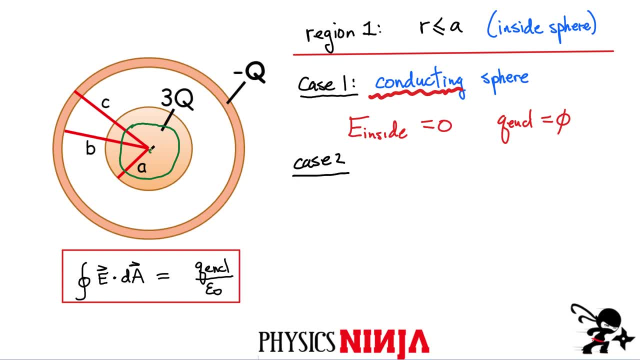 And that's again. it's going to look like a sphere. Mine's a little bit rough looking, but that's okay. And the sphere here has a certain ratio, right, A certain radius. Let's call it radius little r, like this: 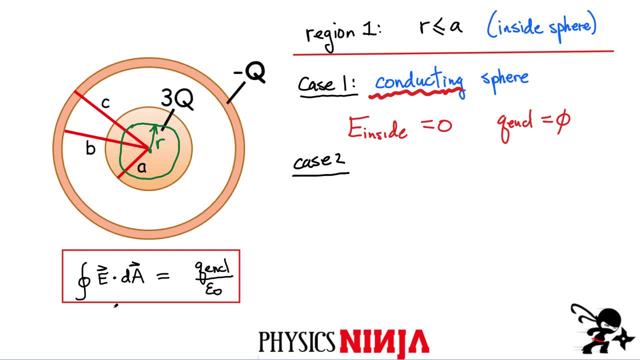 All right. so the question is: how do you apply Gauss's law for this? So, since this is spherically symmetric- actually the left-hand side of Gauss's law is always pretty straightforward, okay. So, first of all, to get rid of this integral, 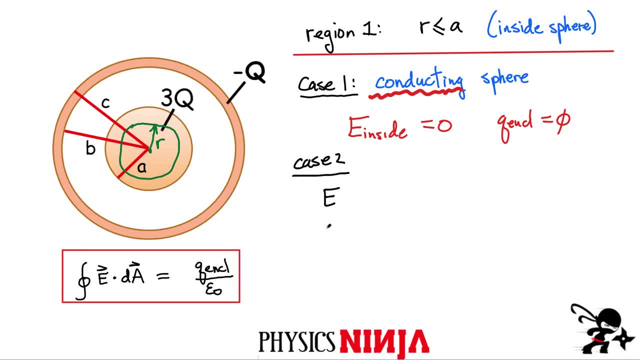 the integral will simply simplify to something like this: It's the electric field magnitude multiplied by the surface right, And the reason that it simplifies is because, again, the electric field produced by any amount of charge inside the sphere is going to be pointing straight out. 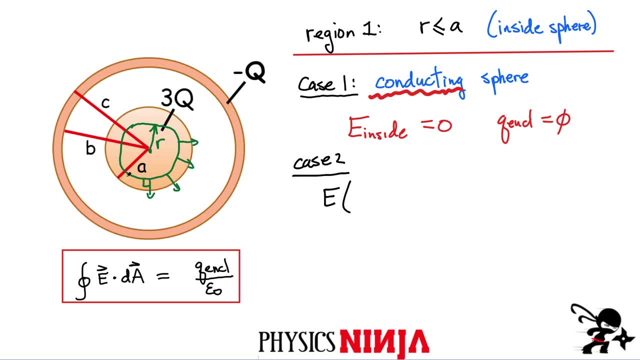 And the area is also right. if I look at the little bit of area of my sphere, that's also a vector that points radially outward. So what we need to do now is simply evaluate what is this total area of the sphere. 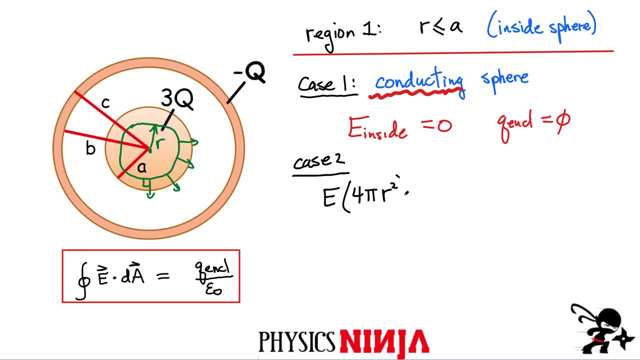 And in this case it's simply four pi r squared. This is a formula for the surface of a sphere that has a radius r. All right, so now we write down the rest of Gauss's law. All right, so now we write down the rest of Gauss's law. 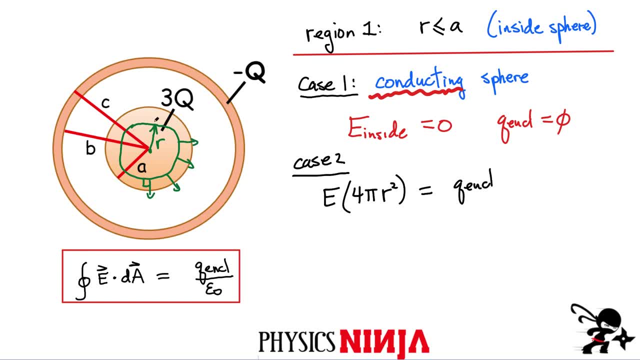 All right, so now we write down the rest of Gauss's law. It's the charge enclosed in this green surface and divided by epsilon zero. All right, pretty straightforward. Now you have to use kind of your judgment here and try to evaluate. how do we find? 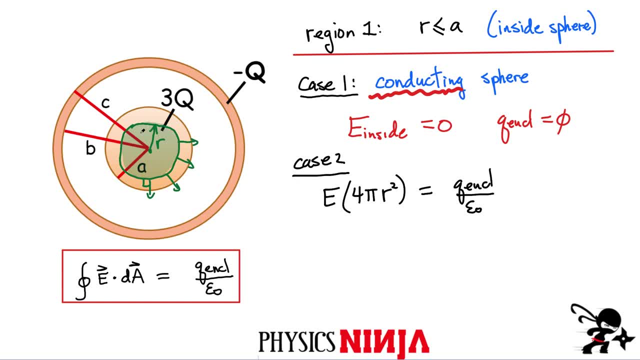 how much charge is inside. okay, Now, it's not equal to three Q because three Q is the total charge, So it's going to be a fraction of the total charge, right? If you think about how much charge is enclosed, let's go ahead and write it down. 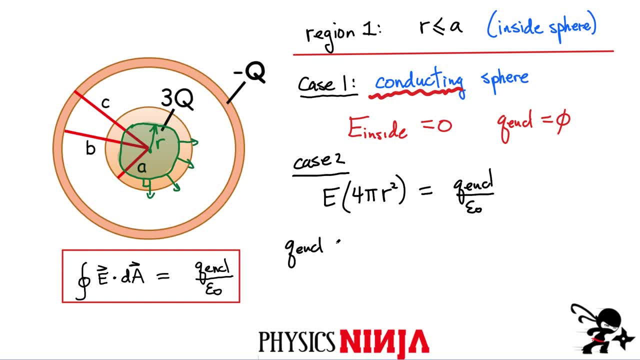 Let me get my marker All right. so we have Q. enclosed is really going to be a fraction of the total charge. Now what you could also do is you could define a charge density which equals to the total charge divided by the total volume. 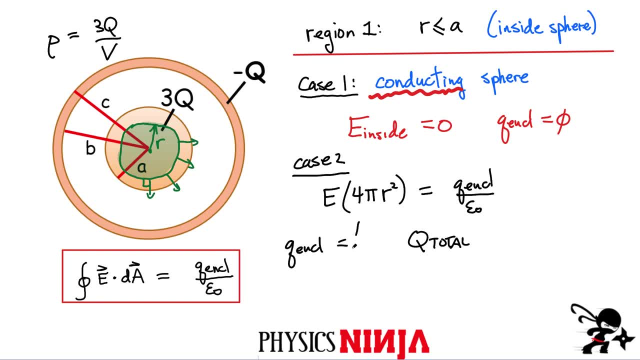 and then integrate over the volume. You really don't have to do that. You could just say it's going to be a volume fraction of the total charge. So this would be the total volume of this sphere, which is four pi R cubed, and in this way it's A cubed right. 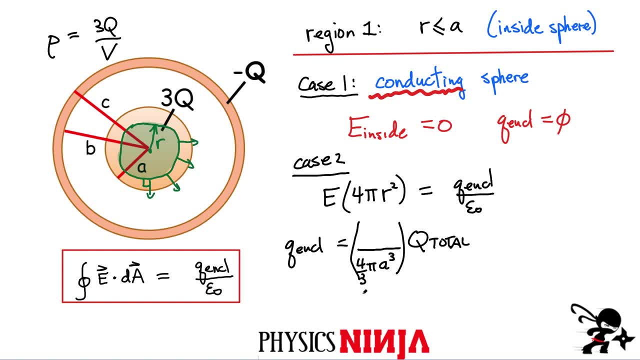 Because the radius of the sphere is A, And now how much volume is enclosed here in this green surface? It would be again four thirds pi R cubed. All right, well, we can simplify this expression a little bit: The four thirds cancel, the pi cancel. 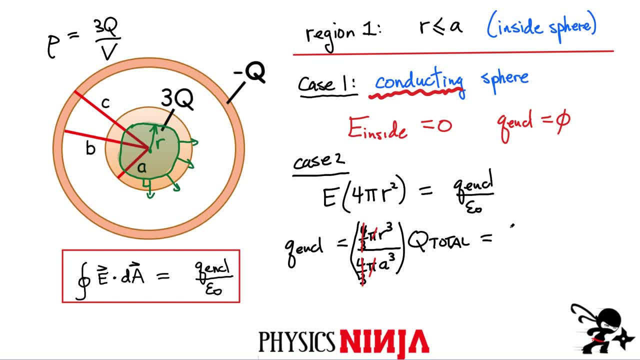 and my total charge is really three Q. So at the end, this here simplifies to R cubed multiplied by three Q. So I've got the three in the front and divided by A cubed. Okay, so now I'm just going to put everything together. 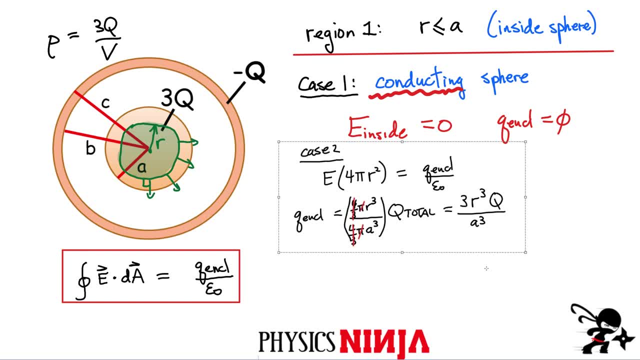 Let me give myself a little bit of extra space here, kind of shrink that down. Okay, so now we plug everything into Gauss's Law. So again, the left hand side was E multiplied by four pi R squared, And the right hand side was Q enclosed. 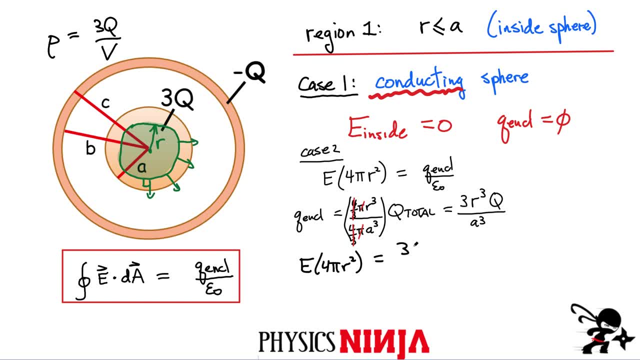 which is my expression here- divided by epsilon zero. So it's just three: R cubed, big Q and divided by epsilon zero, A cubed. Okay, we could simplify a few of the terms here. First of all, you notice you have R squared here. 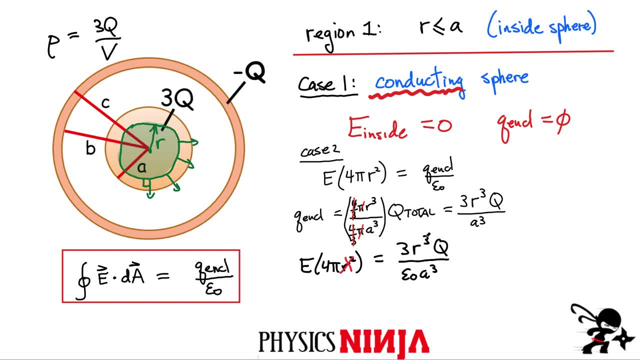 and you have R cubed here, which means you could get rid of two of them and get rid of the two up here. You're still left with one, And at the end you just want one final expression for my electric field magnitude. 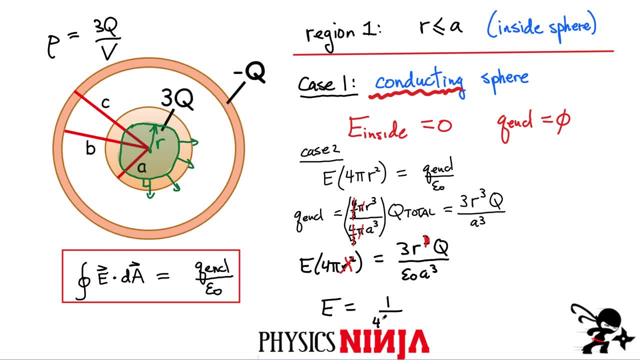 So I bring the four pi down at the bottom so you get one over four pi. epsilon zero. You kind of always have that term right, And and let's look at all the terms that are left. Three Q was the charge, so that term is there. 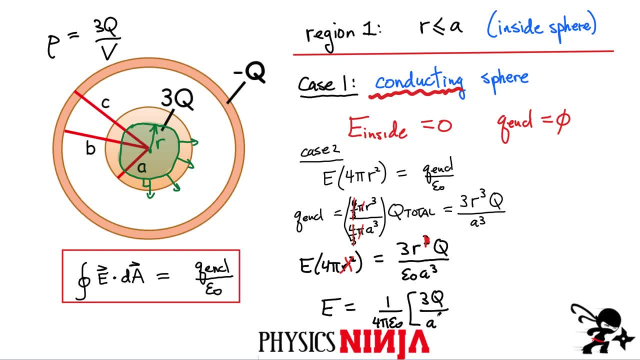 And I still have divided by A cubed. That's just a constant term. That's the radius of this sphere. And then, at the end, I can't forget this R, and this is really, really important, right? So this is, it depends linearly. 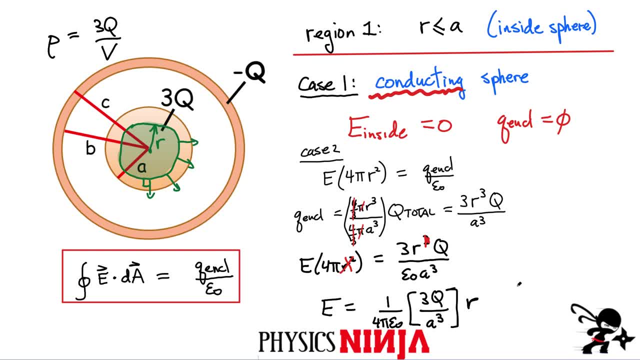 with the distance away from the center. So two kind of really different results. right, If it's insulating and the charge is, you know, it's uniformly distributed, this is what you get, And if it's a conducting sphere, you would get zero. okay. 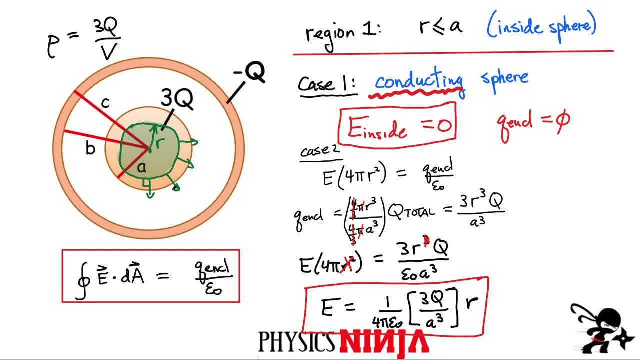 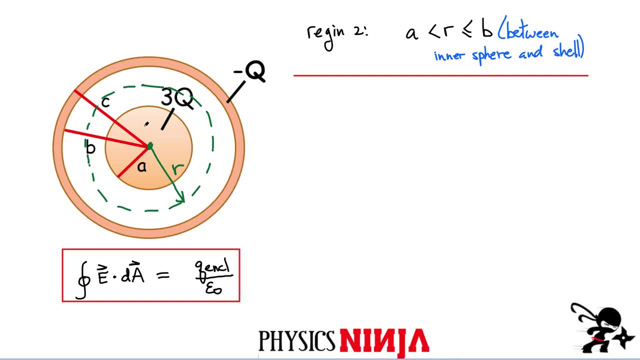 All the way up until the surface. All right, so now let's consider the second region. So for region two now, region two is in this white area, this white space between the sphere and that outer shell, And again, what you first do is you draw a Gaussian surface. 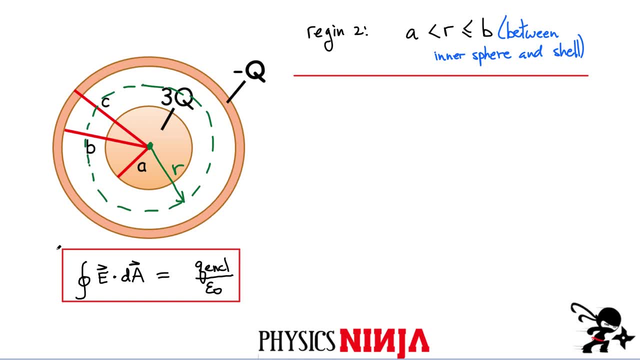 somewhere within that white region. And my goal now is to write down Gauss's law. So again it's, you know, it's, you know, it's, you know it's spherically symmetric. so the left-hand side of Gauss's law. 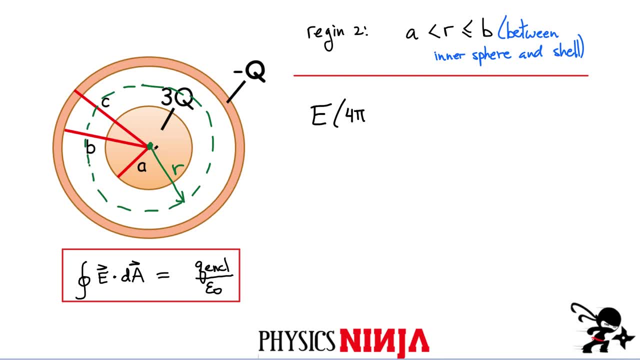 basically always reduces to this four pi, And the area of this sphere is four pi R squared. Okay, that was the left-hand side of Gauss's law. Equals to Q enclosed, divided by my constant epsilon zero. So now you ask yourself how much charge is enclosed? 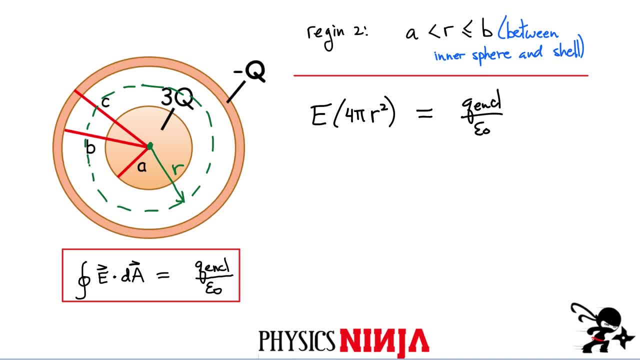 by this shell or by this Gaussian surface, rather, And again, if you have a look at the diagram, how much charge is enclosed? Well, all of this charge that is inside this inner sphere is enclosed right, And whether it's conducting or whether it's insulating. 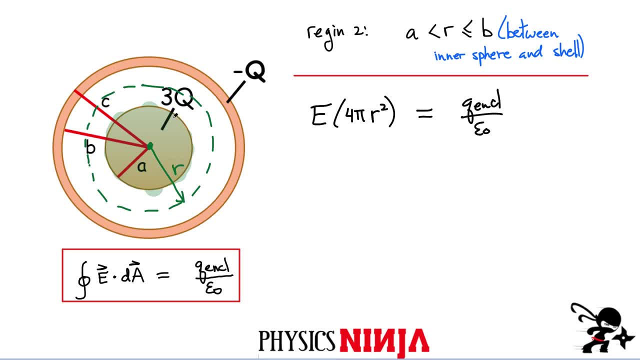 it really doesn't matter, because that total charge was three Q, right? The only difference if it's conducting or insulating, it's the way that the charge is spread out. But really this charge enclosed is always three Q, So I can just go ahead and just write it down. 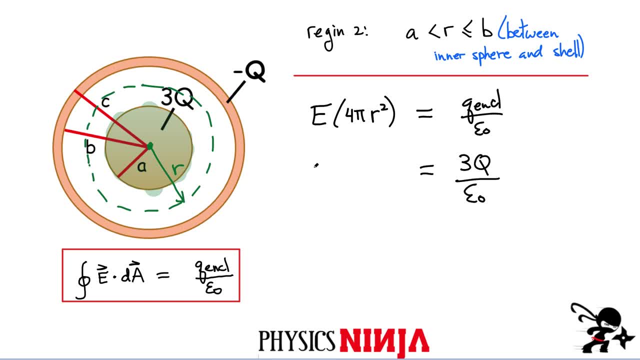 That's the total charge enclosed, divided by three Q, right, So I can just go ahead and just write it down. Divide that by epsilon zero and again just rewrite the left-hand side of Gauss's law here And again bring the four pi R squared at the bottom. 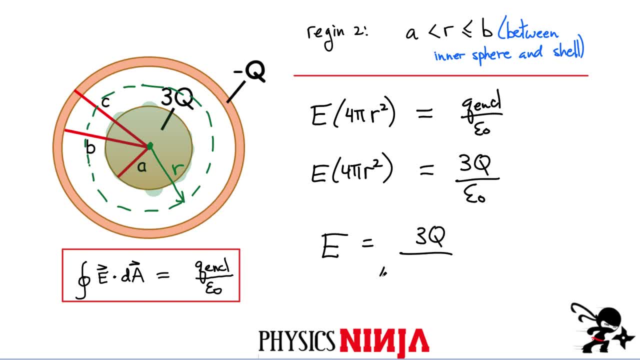 And this is what we're left with. Total charge is three Q divided by four, pi epsilon zero multiplied, or sorry, divided by our squared, like this, All right, So this looks like a familiar expression, right? This looks like exactly the field produced by a point charge. 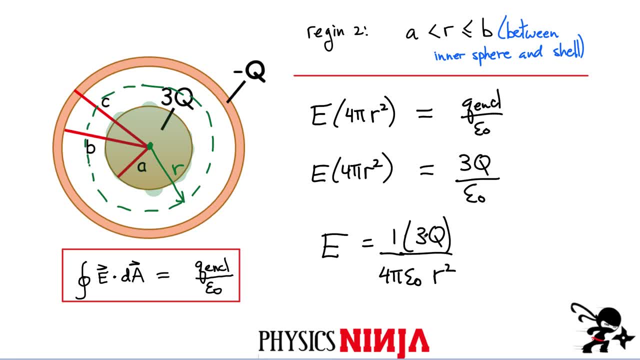 that would have a charge equal to four pi R squared with an equal number, So the whole investment charge equal to 3q, and that charge would all be concentrated at one point right. And if I'm a distance r away, this would be the expression I would use to find the magnitude of the field. 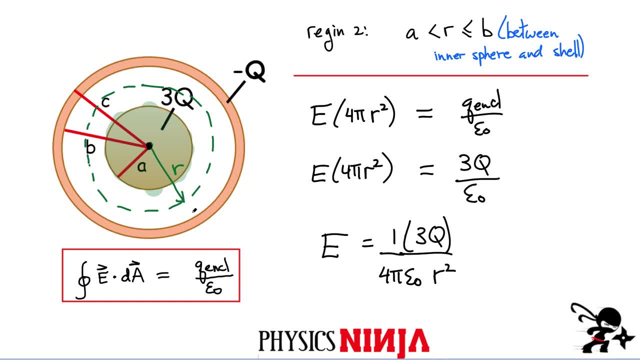 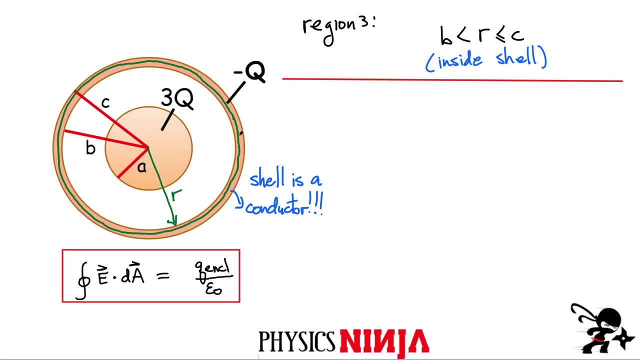 produced by that point charge. okay, Kind of a nice result from Gauss's law. All right, let's consider the third region now. So region 3 now is anywhere inside this outer shell. However, in the statement of the problem, I said something really, really important. okay, I said that this. 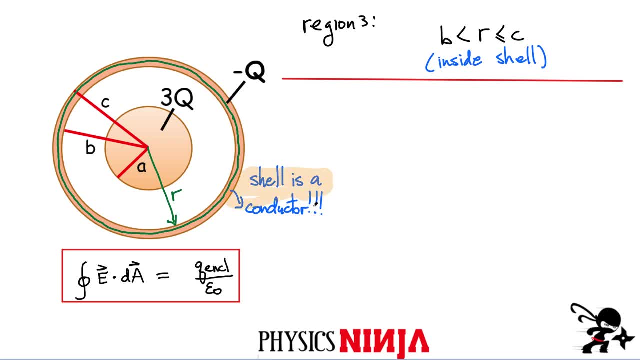 outer shell is a conductor, okay, And this is really, really the key to this problem right here. So if it's a conductor, you should automatically know the field inside anywhere inside this, the field inside the outer shell. let's just write it as e. subscript shell must be equal to zero. 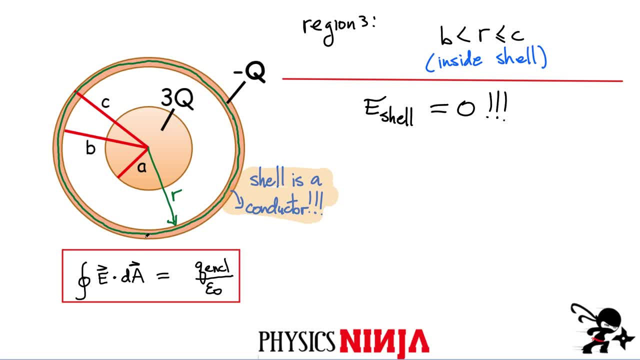 It's a conductor. Now, if you think back of our Gauss's law, well, think about our Gauss's law. What's the electric field in this region? Well, let's write down Gauss's law. The left-hand side of Gauss's law would be e multiplied by 4, pi r. squared Again, this is a spherically symmetric. 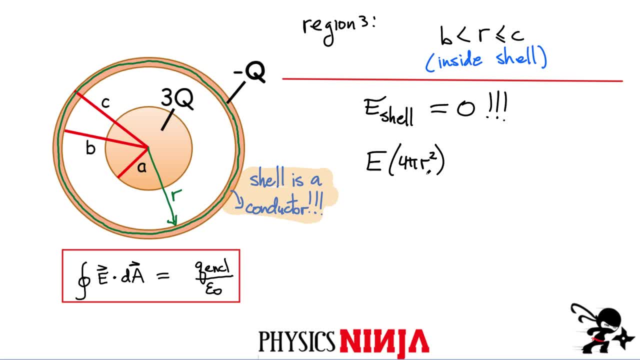 object. so this is how it would look like, and the area of my Gaussian surface over here is 4 pi r squared. Now this has to be equal to q enclosed, divided by epsilon zero. How do we get q enclosed for this problem? Well, let's think about how much charge is enclosed here. 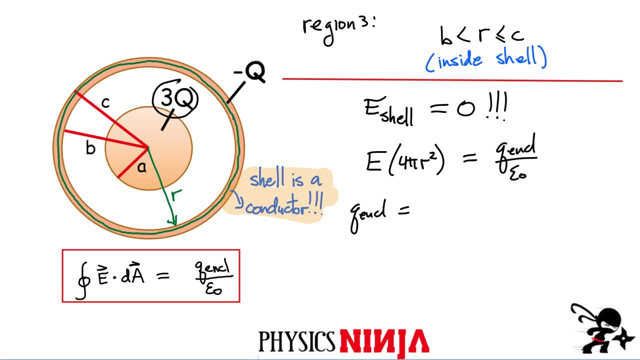 All right, so we have charge enclosed. We definitely have enclosed all of this right, Because my Gaussian surface is out here and I have 3q. okay, But I do require this statement, right? How do I get zero electric field? The only way I can really have zero electric field is if my q. 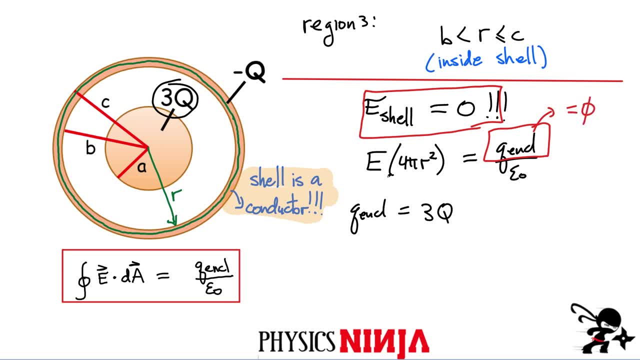 would also be equal to zero. If q enclosed is zero, then automatically the field is going to be zero. So that means that there has to be some charge that has to go on this inner wall of the shell. And now the question is: how much charge goes on this inner wall? Well, we have to add it. 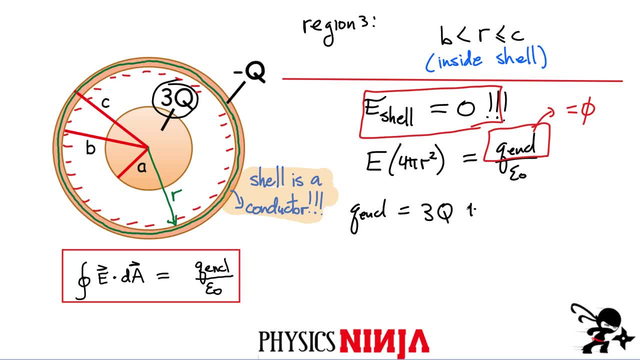 up because it's going to be enclosed by this Gaussian surface. So it's going to be plus q. I'll just write it as inner wall, Okay. so at the end of the day, we do require that the q enclosed over here is equal to zero. 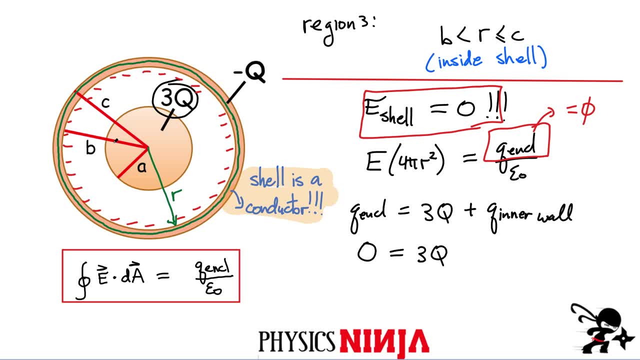 And the only way you can have this, because I do have the 3q enclosed from the sphere. that means that the inner wall, q inner wall, must be opposite of whatever the total charge is from the sphere. So at the end of the day I find that the only way I can have zero electric field. 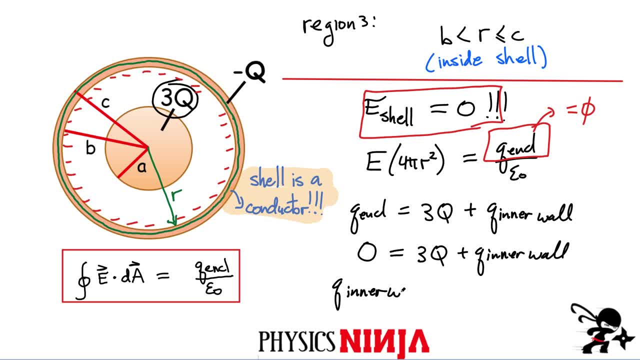 inside this conductor is if the charge on this inner wall is equal to negative 3q. This is a requirement And this will ensure that the total charge enclosed is going to be zero, And that is going to force that electric field to also be zero. Okay, so let me go ahead and write this: 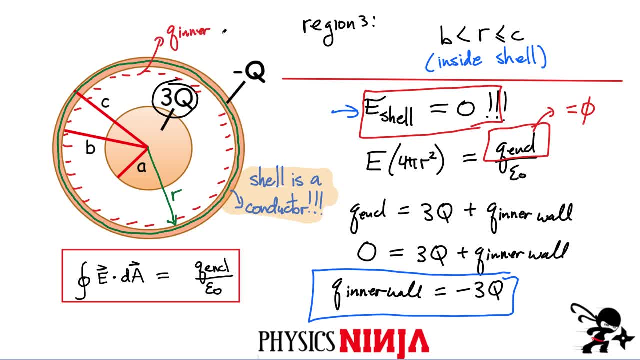 So q inner wall must be equal to negative 3q. All right, so this way you add up And if you do this you're going to get, let's say, negative 3q. add negative 3Q to the plus 3Q of the sphere and you're going to get zero total charge. 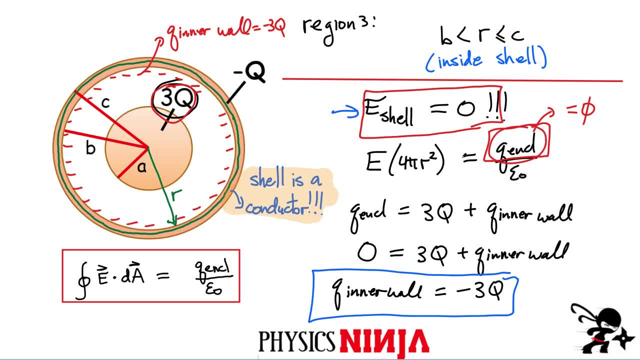 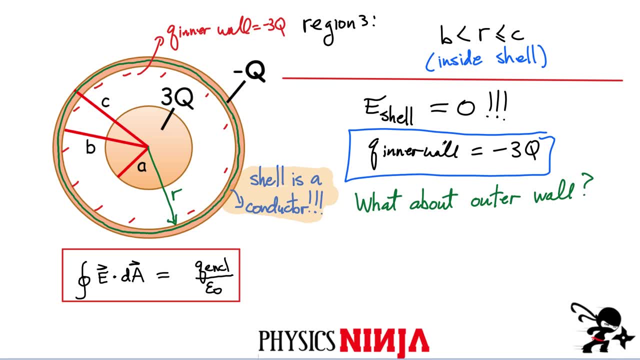 enclosed. If I have zero total charge enclosed, I'm going to get zero electric field anywhere in this region. All right, so the next question we have to ask ourselves is: well, if this inner wall has negative 3Q, like we calculated here, what about the outer wall, right? How? 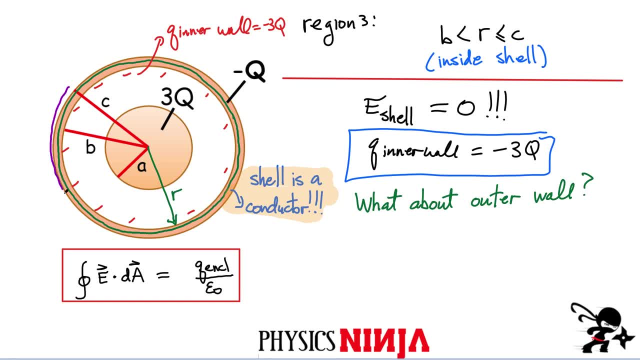 much charge is actually on this surface over here of that shell And in order to answer that, you simply have to look at the total charge of that conductor In this problem. I said that the total charge of the conductor was negative Q. All right, so this is kind. 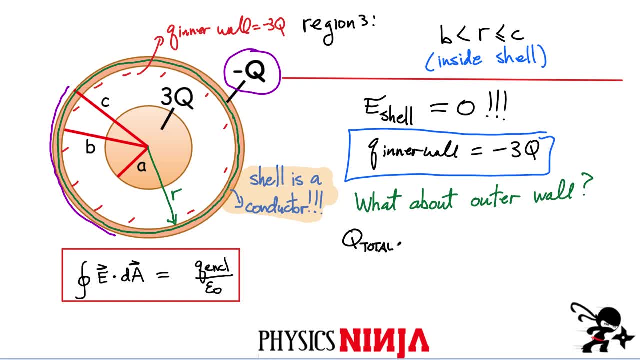 of what it looks like, right? So Q total for the shell has to be equal to whatever is on the inner wall, inner. I'll just write it as Q inner plus whatever is on the outer wall. Okay, Okay, And the total charge of the shell is given by this number negative Q, right? This is? 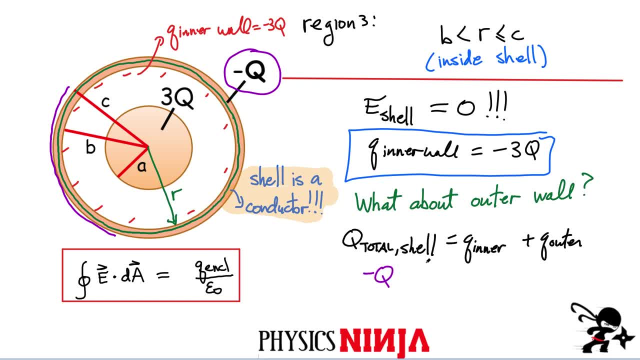 what we had. This was negative Q. We just solved for what was on this inner wall. The inner wall, we said, was negative 3Q, So plus Q outer. So at the end now you just bring the negative 3Q on the other side. You're left with that, the charge on the outer surface. 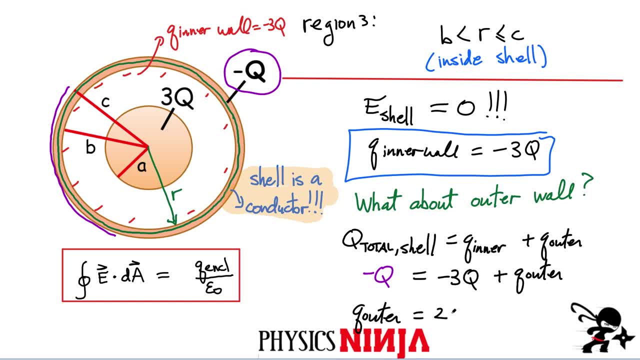 okay, Charge on the outer surface must be equal to 2Q. You have no choice. You have to have conservation of charge. So if I put negative Q on here, that means that on the inner wall I'm going to get negative 3Q And on the outer wall I have to have plus. 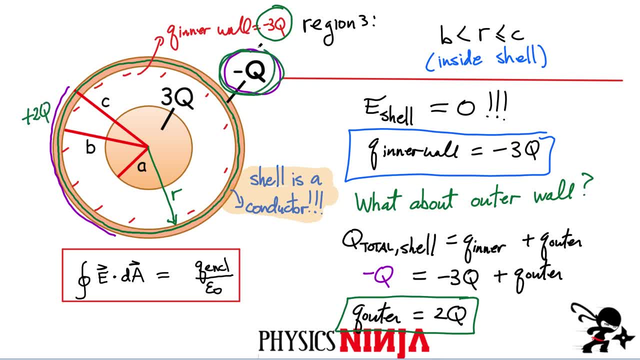 2Q. That's the only way that both of those are going to sum up to equal to the total charge on the shell. okay, Because negative 3 plus 2 gives me negative 1, which is what I said in the problem statement. okay, And you have this distribution of charge because we do require that. the field 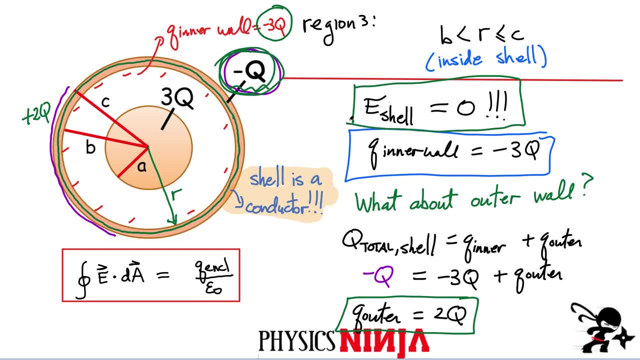 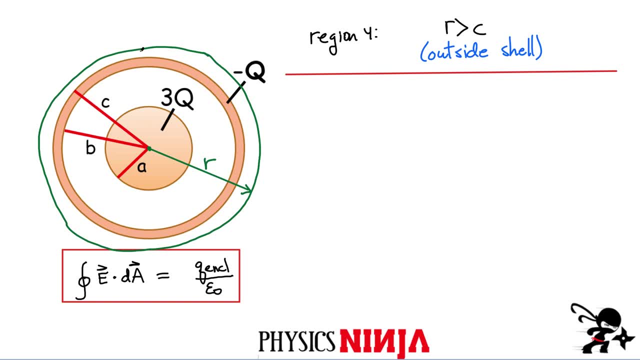 is equal to zero everywhere in the shell, because it's a conductor. Alright, let's go on to the final region. Okay, so this is now region four. What I've drawn is a Gaussian surface. It is on the outside, because this is where I want to evaluate. 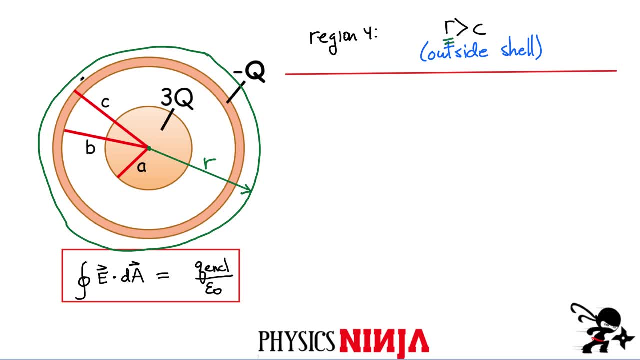 the field. I want to evaluate it when the radius is bigger than C, So I want to be on the outside of that conducting shell. Alright, again, we apply Gauss's law to this problem. we want to look at the field dotted with the area. 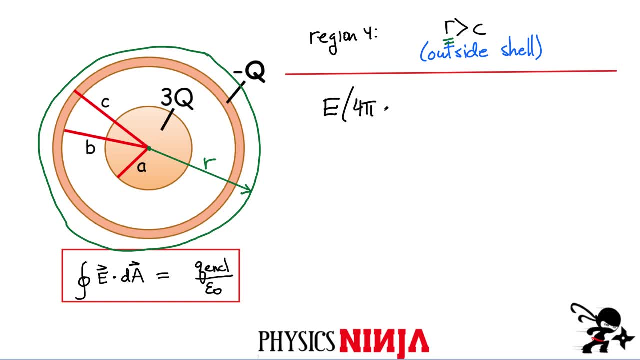 It's a surface, so the area of that sphere is four pi r squared. Always the same thing for spherically symmetric objects. All right, this must be equal to again, how much charge is enclosed by that surface divided by epsilon zero. 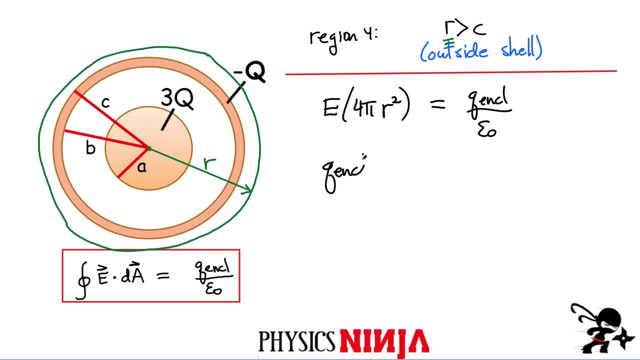 Well, now let's look at what is Q enclosed for this problem. Well, number one- I am enclosing this entire sphere, right? I definitely have all of that charge. So if you go ahead and write this, you have to have definitely plus three. Q is enclosed. 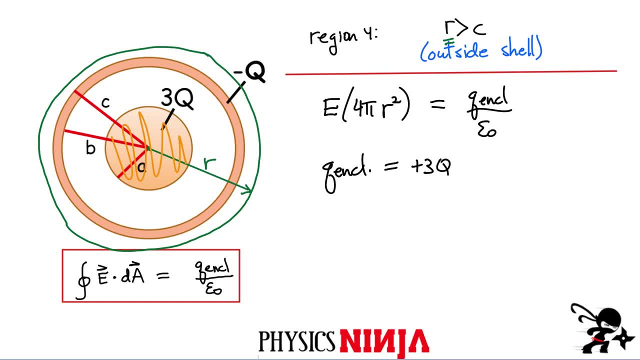 by this Gaussian surface. What else? I am also enclosing all of the charge that is on the shell, And all of the charge on the shell is well, it's negative Q. So at the end, what I have is two Q. 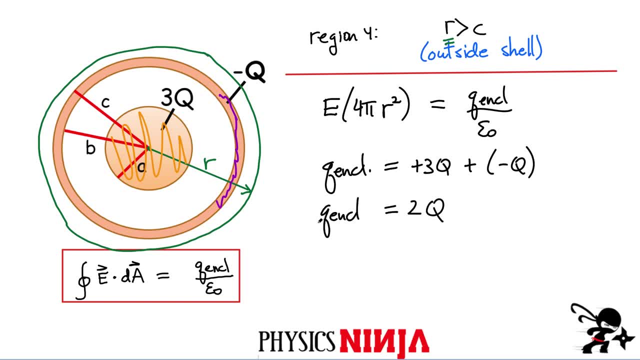 This has to be the total charge enclosed by my Gaussian surface in this case. So we go ahead and we substitute that into Gauss's law. So you get E. four pi r squared Must be equal to two Q divided by epsilon zero To get the final expression. 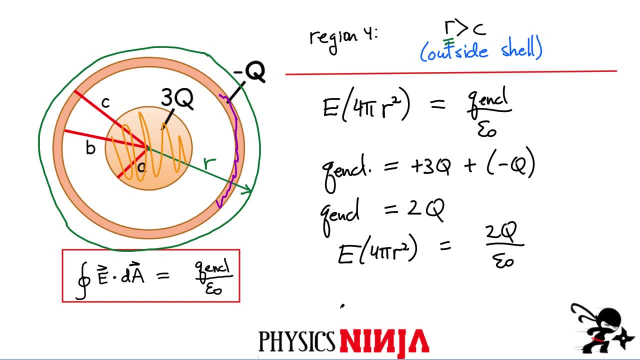 you just bring all of this term in the bracket here down in the denominator on the other side. So you get two Q divided by four, pi epsilon zero and over r squared Again. if you look at this result, this would be the result that you would get. 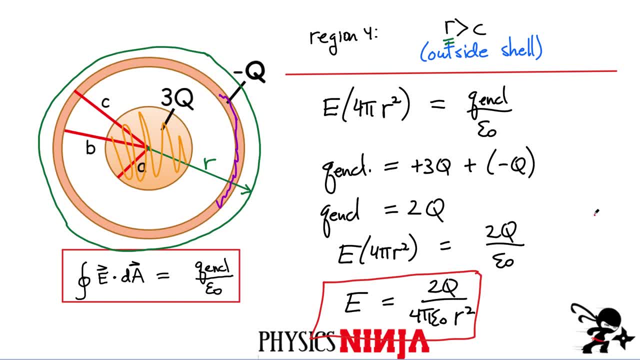 if you had a point charge And if the point charge was equal to two Q, you would get a point charge And I was a certain distance r away from that point charge, right? This is if I'm evaluating what is the field at this point. 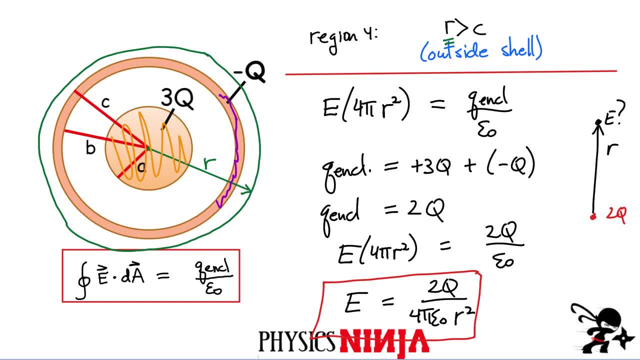 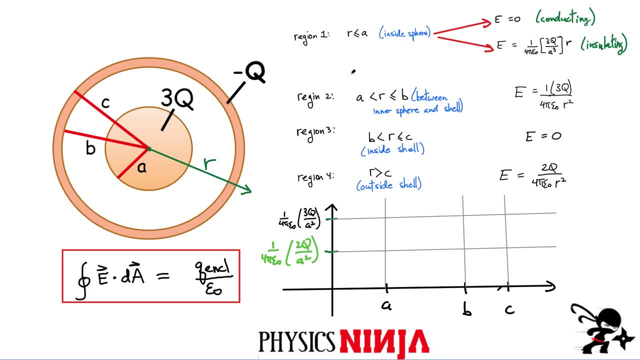 I would get the exact same result. okay, And that's kind of obtained from Gauss's law this way. So here's a summary of the results that we obtained. Let's try to make a sketch now. So for the region, from what I'm plotting here, 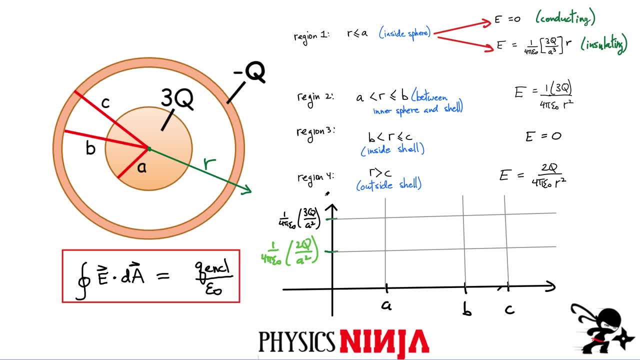 is the magnitude of the electric field. Just write it as E here on the y-axis, And I have the distance r on this x-axis, And again, let's draw the different cases. So the first one we're gonna do is: well, if it's a conducting sphere, 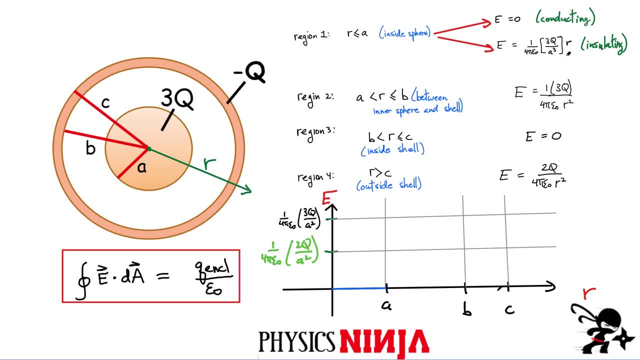 then you should have zero here. Now. this other one is: if it's insulating. let me put in a different color over here. It should be a linear relationship and it should go all the way to the top over here. Okay, so the field grows as I get away from the distance. 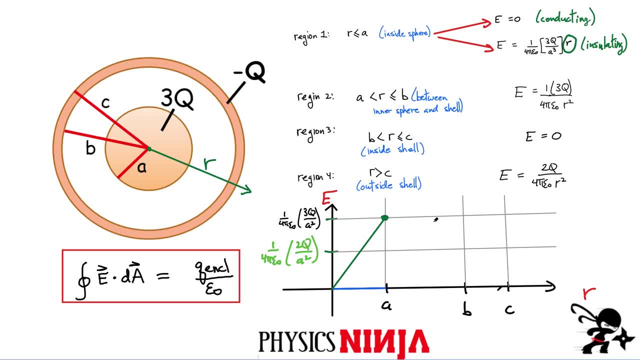 because I end up enclosing more charge. All right, and let's do the second region. The field is kind of the same. It starts off in both cases up here and it rolls off as one over r squared, So it should look something like this over here: 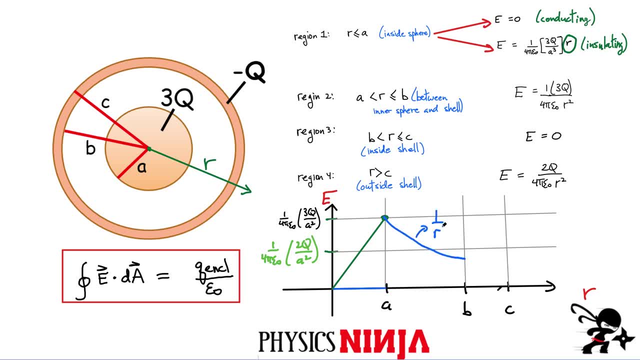 All right, it should roll off here and this is like a one over r squared dependence. All right, and what about the next part? This is the region here in the shell, between B and C. So in that case, that case is pretty easy to draw. 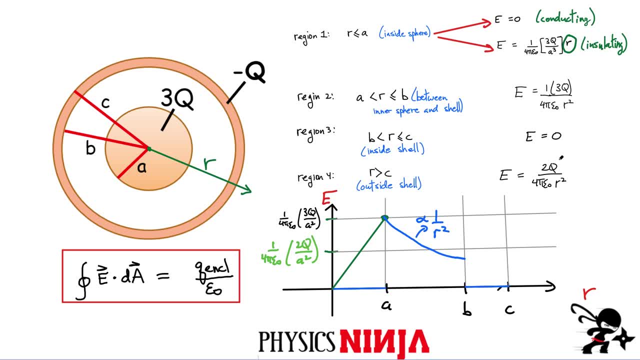 It should just be zero because it's a conductor And in the last region, this is a conductor In the last region. again, it should probably start at some value. over here It's gonna be lower than this because I'm further out. 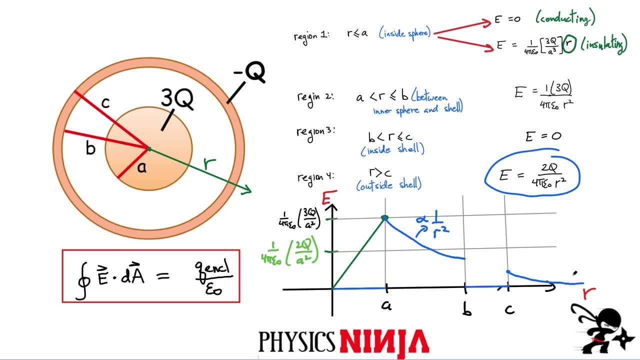 And again it's gonna roll off as one over r squared. Again, this is proportional to the distance squared. All right, this is kind of what it looks like Again in these regions. here you could have zero because it's a conductor. 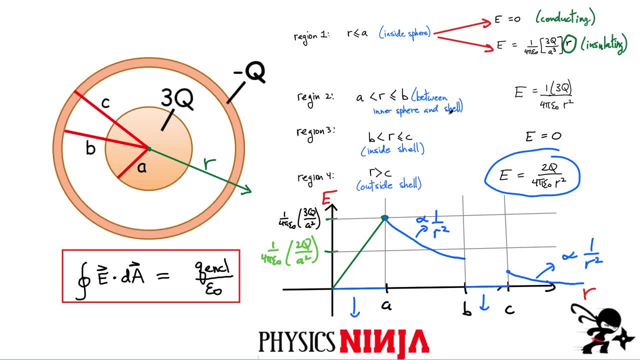 And again it depends on the case here that I looked at, but this is what a sketch would look like for this electric field. All right, thanks for watching folks. Hopefully you understood it and you become a better problem solver.